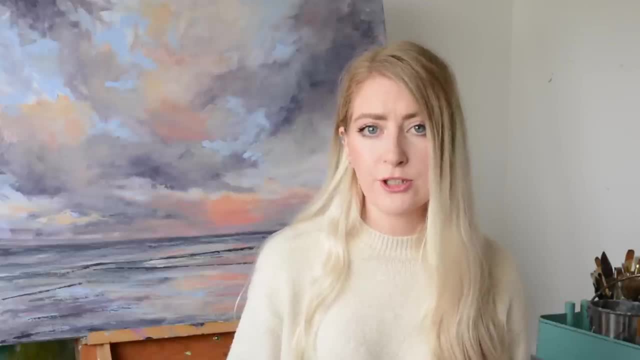 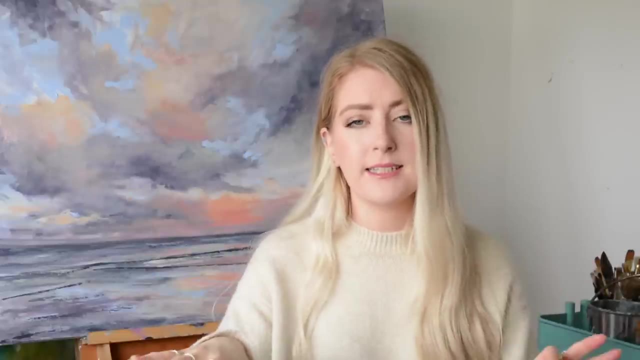 might take a lot longer to dry. If you're just going to go and grab some lunch and you don't want your paints from drying out on your palette, you can just pop a layer of cling film on top of your paints and just dab it down in all the right places, and then, when you come back, you should just be able. 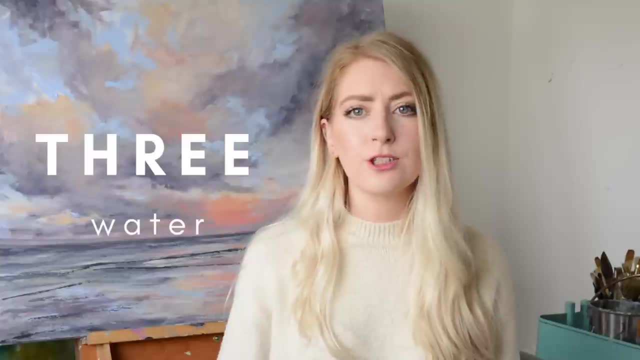 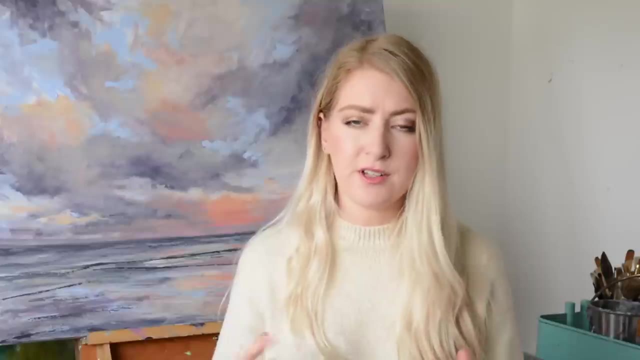 to peel it off and it will be exactly how you left it. Another tip is not to use too little or too much water. I feel like this is really difficult to get right when you first start acrylic painting, and it's only through time, really, that you can really learn how to do it. 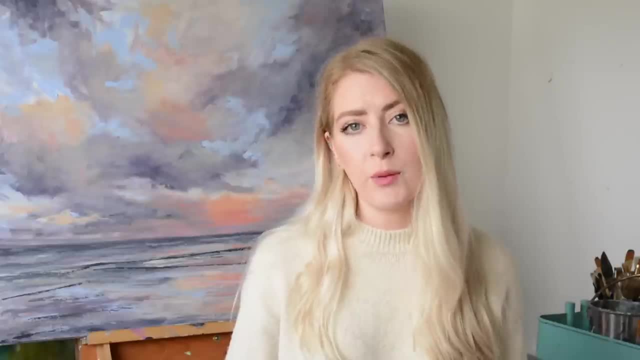 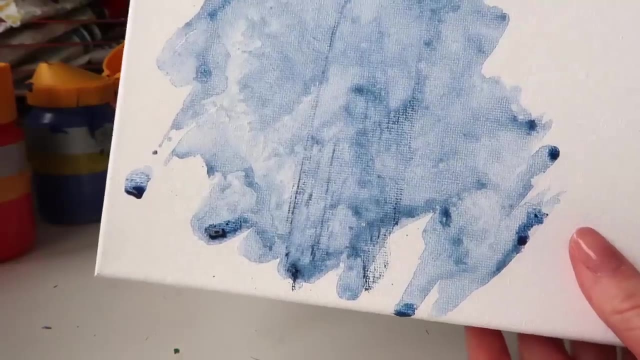 I'm going to show you how to do it. For example, we might be using so much water that it's almost pooling up on the canvas, and then, when it dries, you might totally be able to see the canvas underneath and almost like a coloured canvas, and that's definitely not what we want. 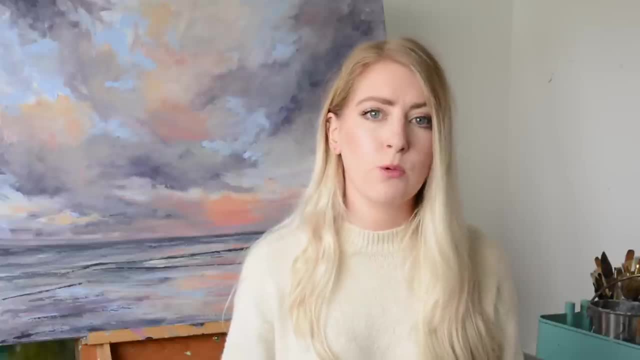 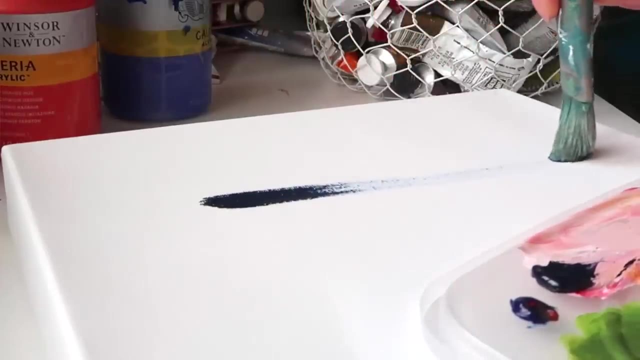 If you do like to use a lot of water in your work, then I would really suggest trying watercolours instead. Or, on the other hand, we might be using so little water that our brush strokes are just really struggling to get across the canvas, and it makes blending very, very difficult. 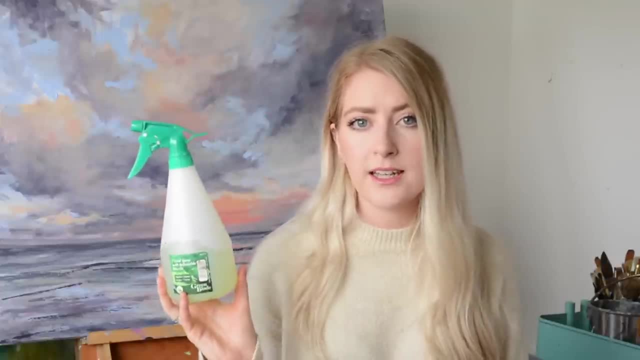 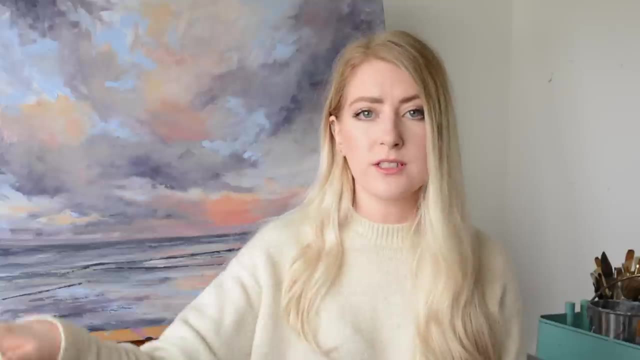 I usually lightly spray my paint. I lightly spray my canvas with this water and that just helps the paint to glide across it more easily. It also means that I don't have to add much water to my paints on the palette. So once I've done that, I will then wash my brush out in the water, just nice and clean. 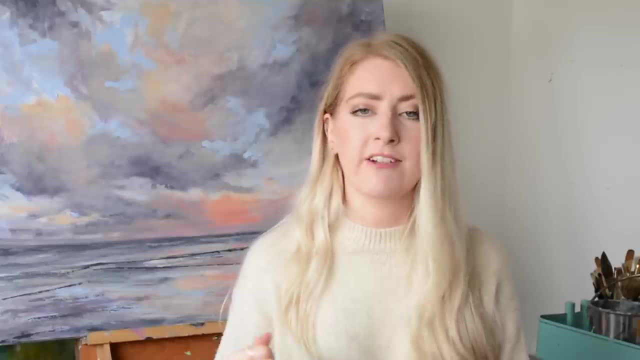 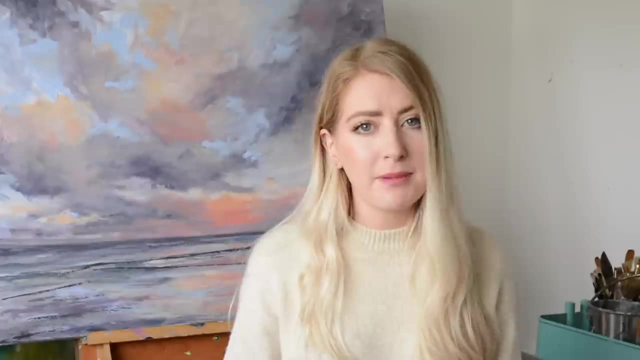 and then dab it lightly on the towel and then go straight in with my acrylic paints, And usually for me that is just the right amount. Tip number four is palettes. There are some amazing palettes that are either really really cheap or even free. 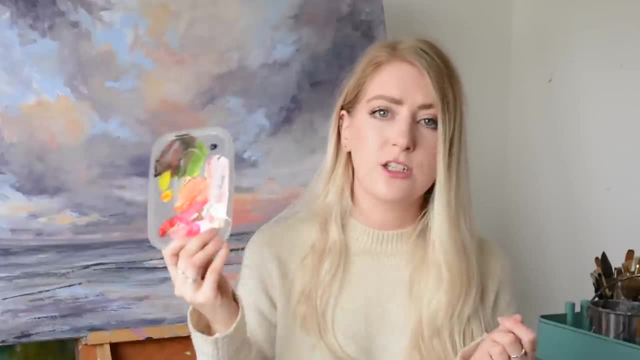 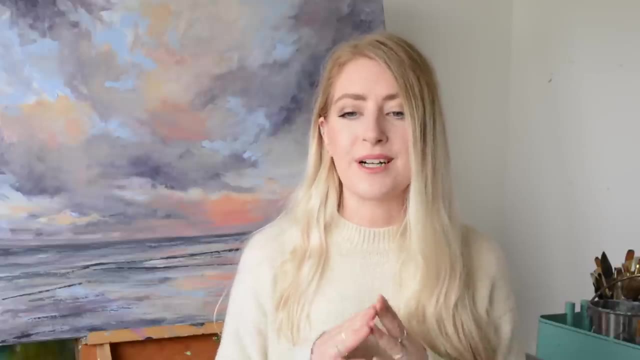 For example, this is one of my favourite palettes And this is actually the top of a Chinese takeaway lid. Another really good option is a glass kitchen chopping board, And I know that sounds really weird, but it's actually very, very similar to the glass palettes. 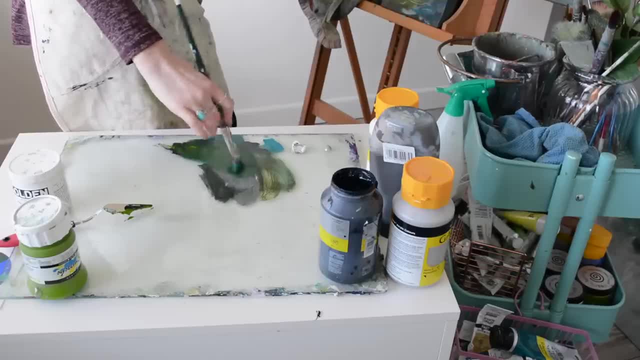 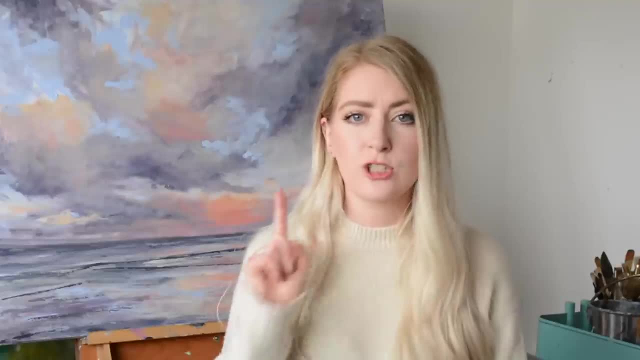 that are out there for like £40 or more. So it's a really, really good option if you're slightly on a budget but also you really want something that is going to really be good and last you for a really long time. Just one quick note: if you do want to buy a glass chopping board, then make sure it's. 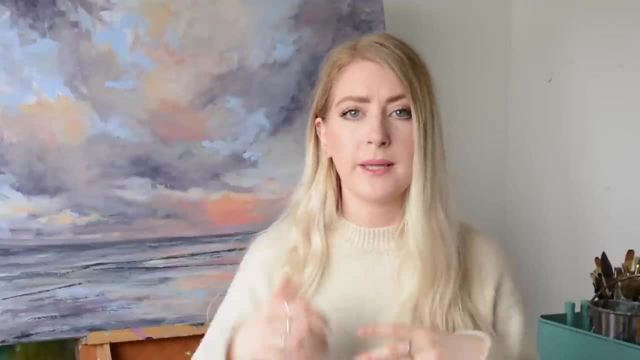 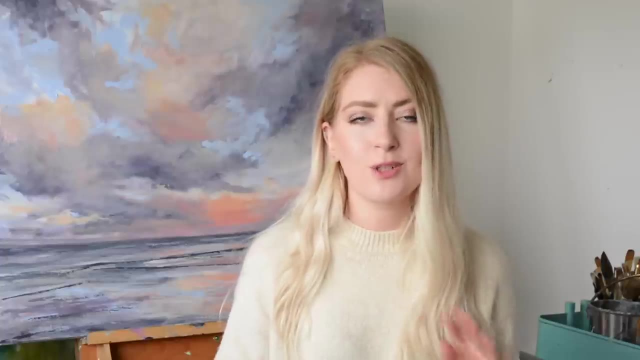 not got any sort of ridges in that the paint can get stuck into, because that will be a nightmare to clean. Tip number five is to build up textures with layers, So sometimes we might feel like we want to sit down and do a whole painting in one layer. 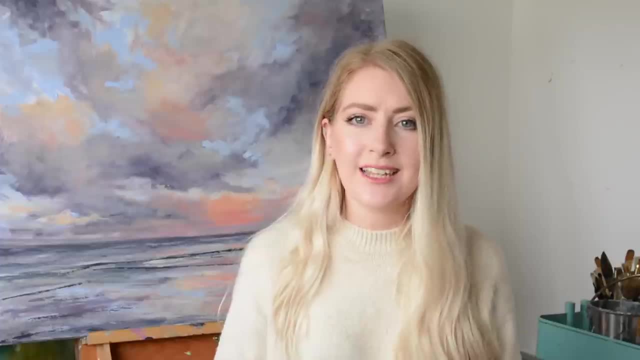 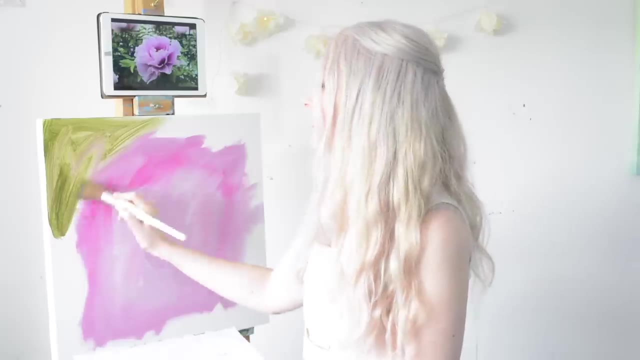 and then it to be finished. But in reality, the more layers a painting has, the more depth and just sort of the more 3D that it will look. If you're unfamiliar with the concept of layers, then it might be really handy to check out. 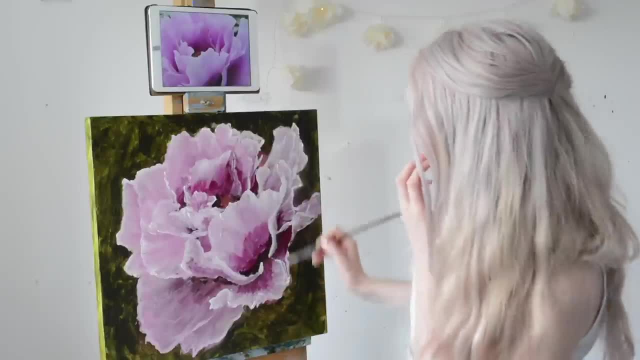 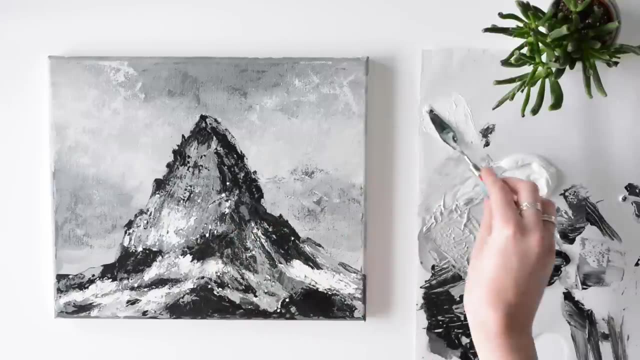 one of my tutorials and you can see the process of that happening and how it ends up to an end result. So again, I will link those in the description box if you've not already seen them. And you can even use a palette knife. They build up really interesting textures, especially in the outer layers, and this can. 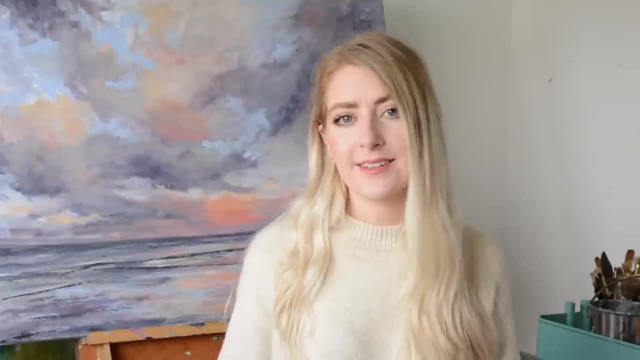 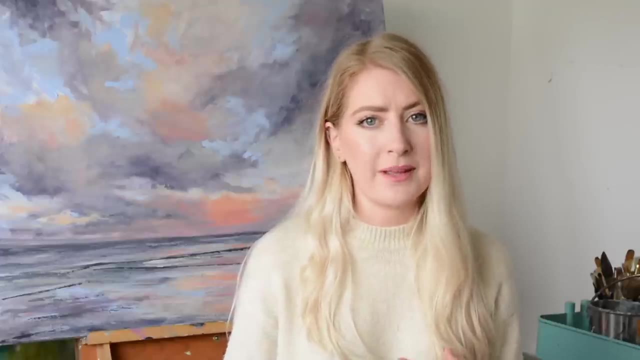 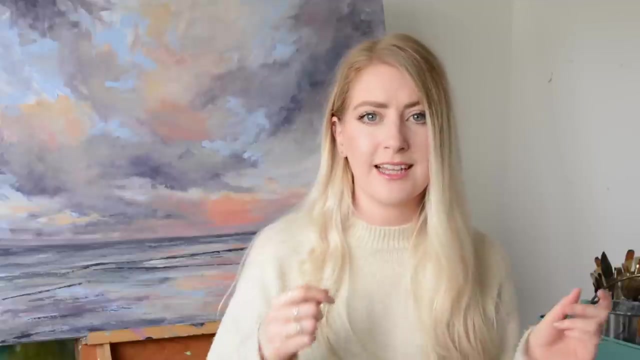 really just add a different dimension to your artwork and make it really unique. Tip number six is to blend and mix colours separately and not to batch mix colours. So in more amateur paintings you will see sort of the blanket colours and it's almost like they've sat and batch mixed three or four different colours and then just coloured. 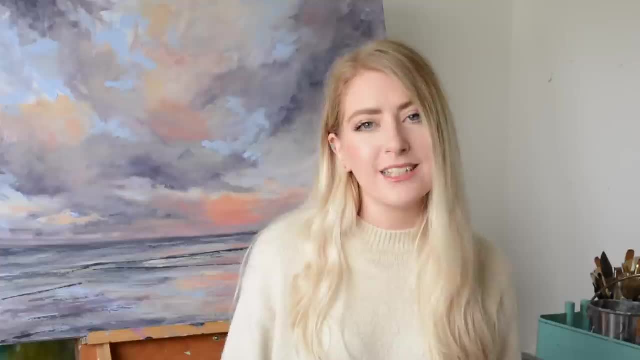 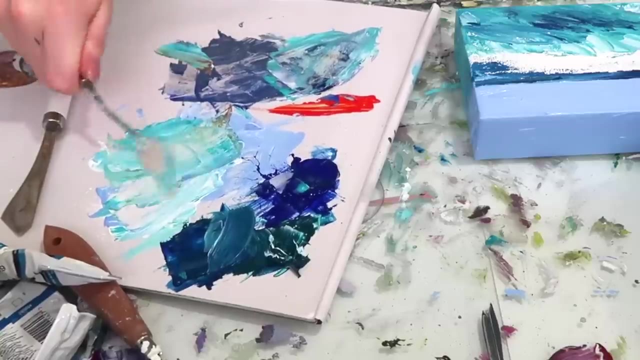 the painting in A little bit like a paint by numbers. This can make it look really 2D and it just doesn't quite like lead your eye in. So instead of batch mixing colours, mix them as you need them and really look at your 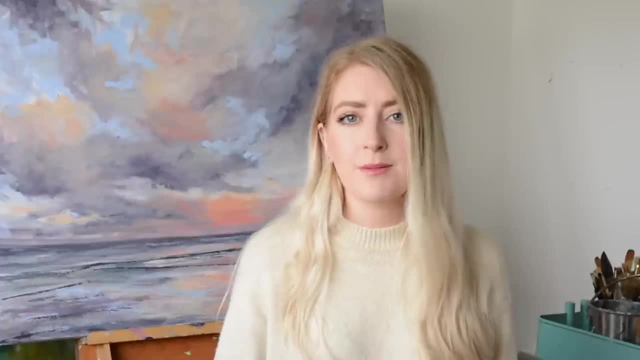 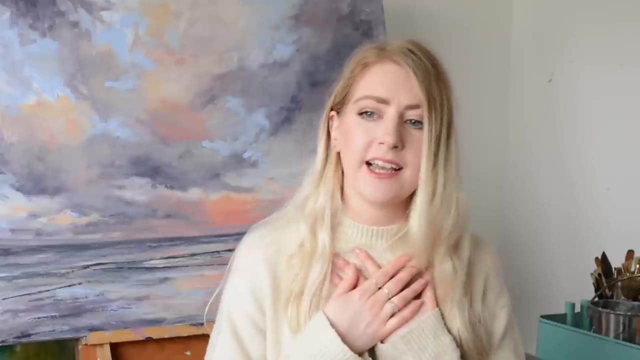 reference photo to see exactly what colour it is that you need to try and make. Tip number seven is to choose your weapon wisely. Choosing a brush is a really personal decision and what I might like or another artist might like, you might not personally get on with. 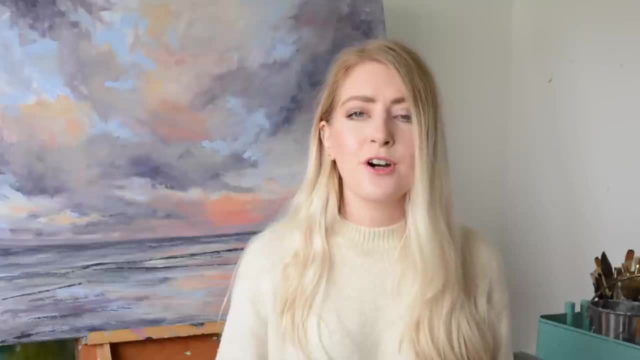 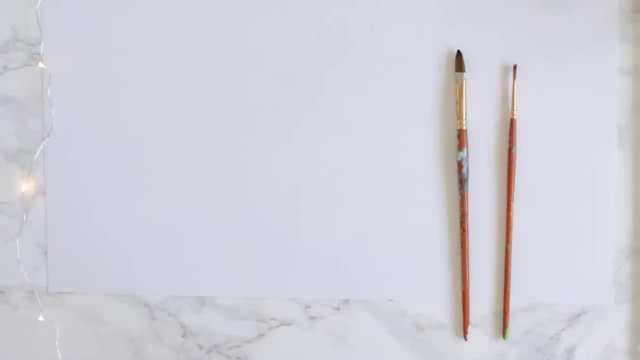 So it's really worth trying a few different shapes And for a beginners toolkit, I would really really recommend a large flat brush, a medium filbert brush and a small round brush. So I've got a few different brushes here And these are nice, different, various shapes and sizes that can really give you a feel. 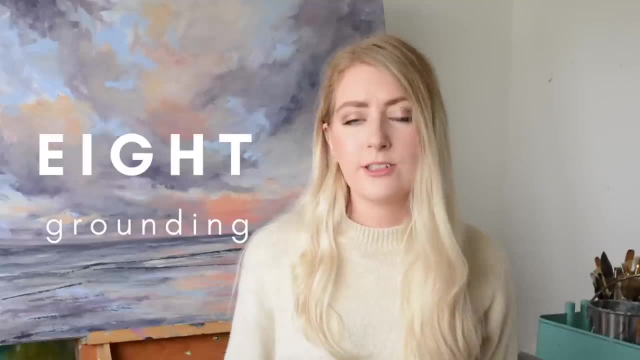 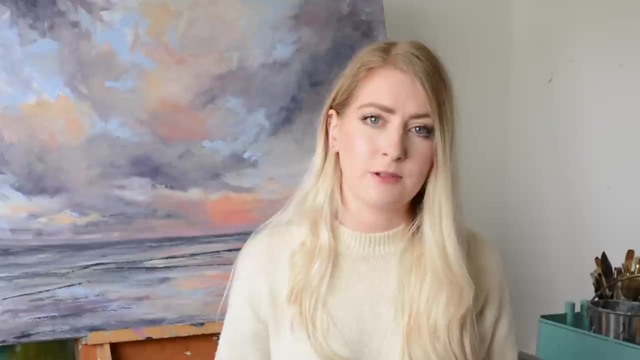 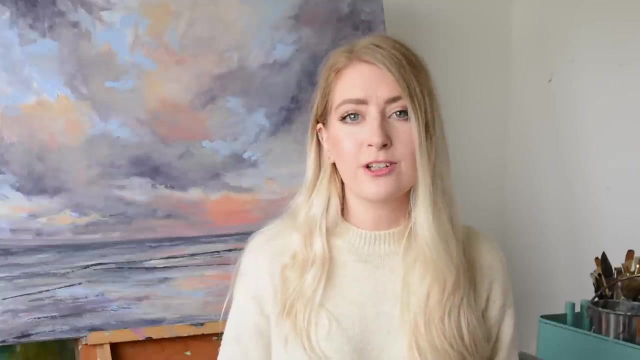 for what you will like to paint with. Tip number eight is to ground the canvas. Now, not every artist likes to do this and I only do it sometimes, but it can really really help when you're sort of learning the painting process. It can end up with a much richer painting, full of texture, and it can help with colour. 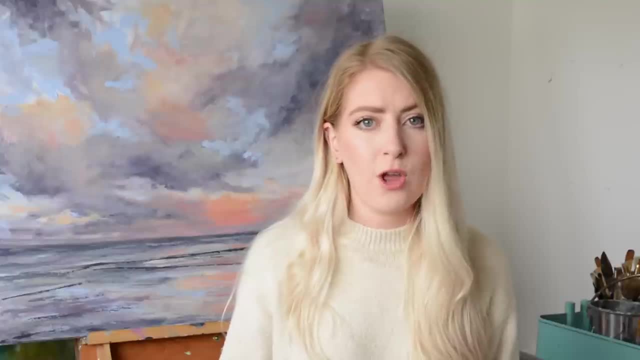 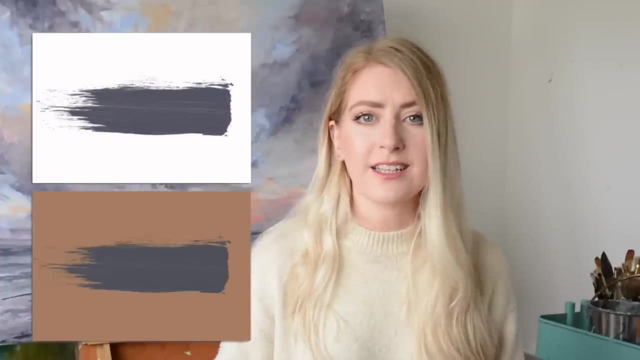 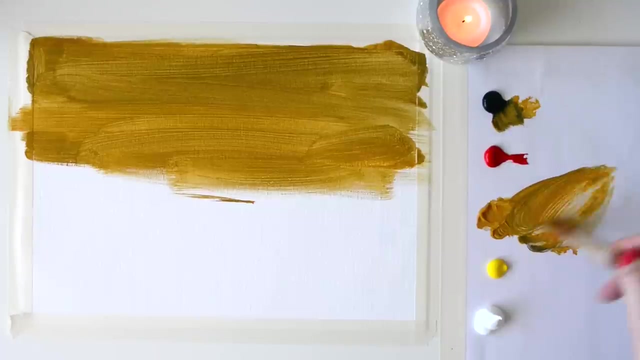 choices as well. Having a plain white canvas can really throw off when you're using colours and it can actually make sort of a medium colour. So if you're painting a blue seascape, you might want to use a really thin layer of colour, and some artists like to use yellow ochre, some like to use a burnt umber, a raw umber.